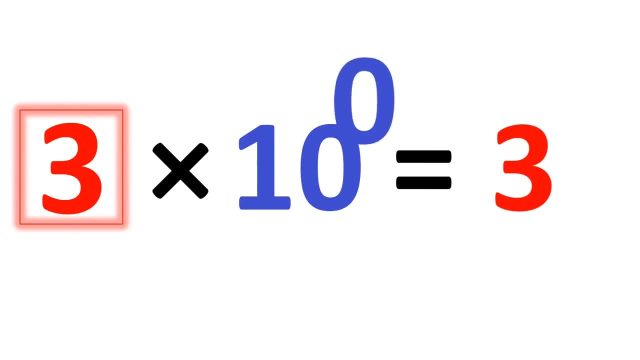 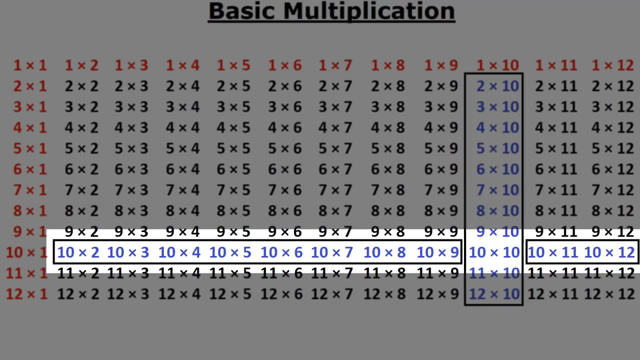 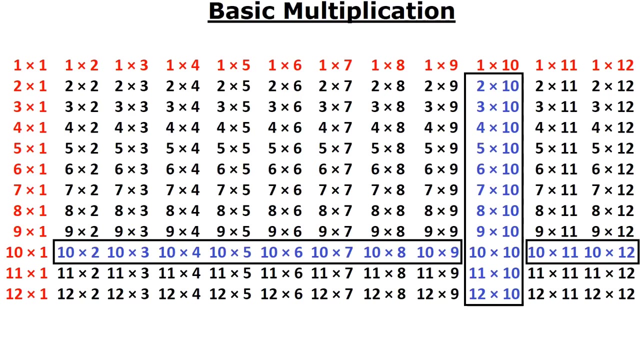 3 x 10 is 3, with an added 0,, etc. You also know the reverse. You also know 10 x 2,, 10 x 3,, 10 x 4.. So now, from those two simple rules, you now have learned 44 multiplication. 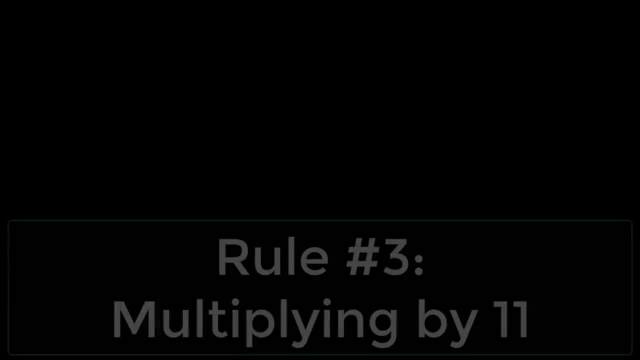 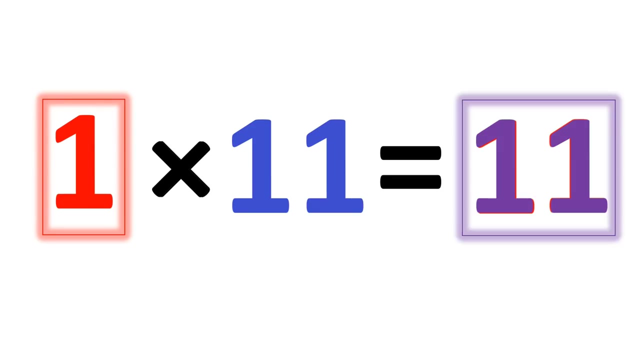 tables And now you have 100 remaining. Here's the third easiest rule: Multiplying times 11.. 11 times a single digit, That digit just duplicates itself. What does that mean? It means 2 x 11 is 22.. 3 x 11 is. 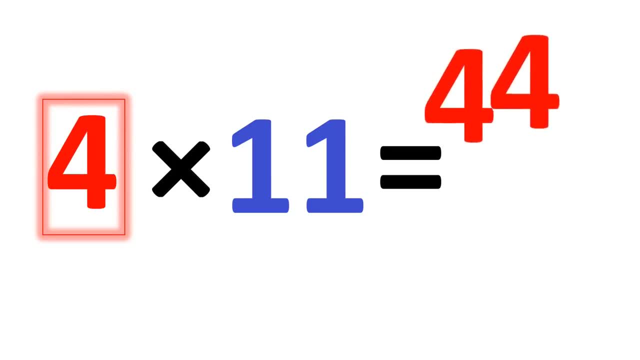 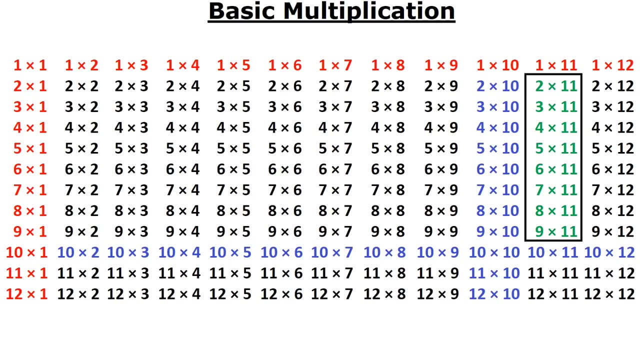 33.. 4 x 11 is 44.. 5 x 11,, etc. You also know the reverse: 11 x 2,, 11 x 3,, 11 x 4.. So from these three simple rules- just three simple rules- you've actually learned 60 multiplication. 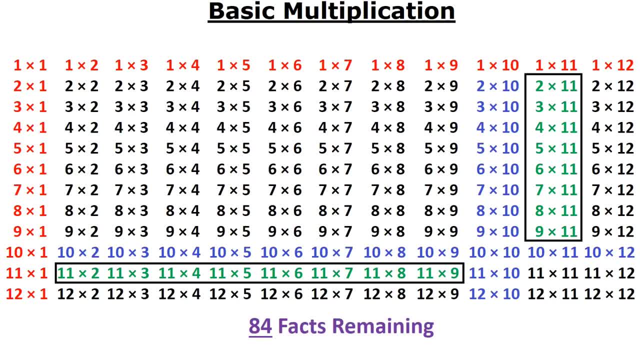 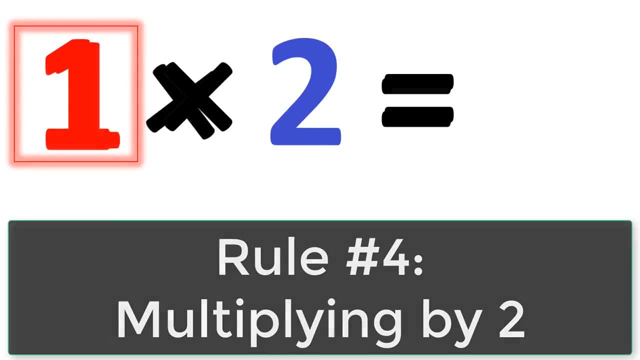 tables And you only have 84 remaining. So from these three simple rules, you've actually learned 60 multiplication tables And you only have 84 remaining From three rules, and these are the easiest rules. Next one is multiplying anything times the number 2.. There are two things you can do. 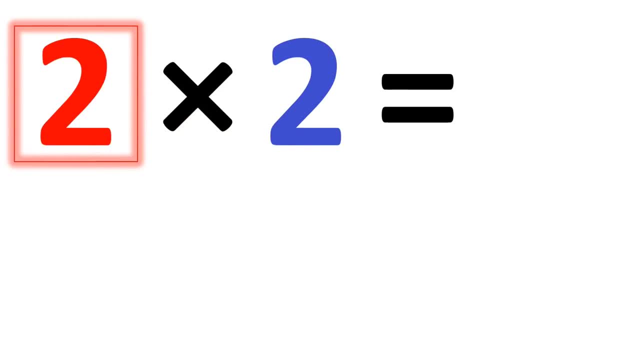 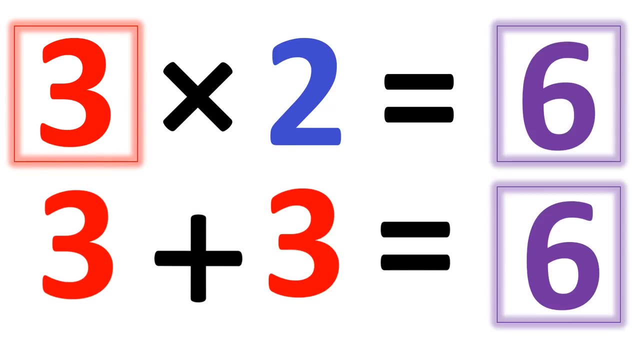 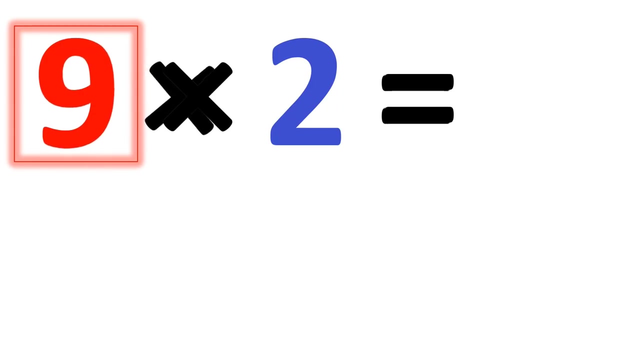 there, First thing you can do is you can double the number, Because 2 x 2 is the same thing as 2 plus 2.. 3 x 2 is the same thing as 3 plus 3, etc. Well, if you forget some of your basic addition, there is a. 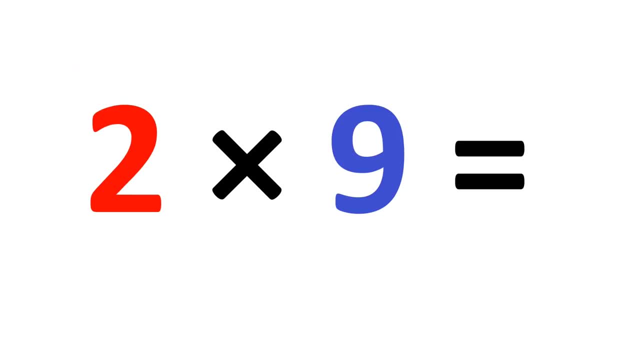 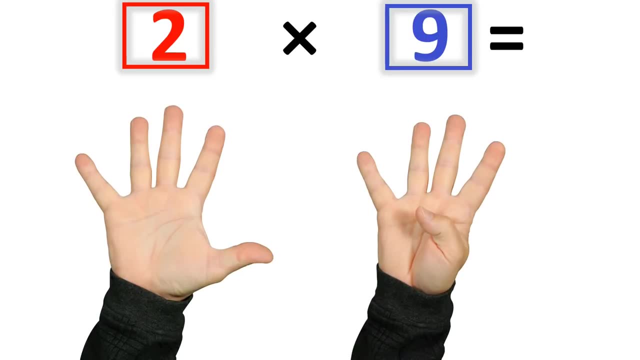 backup method. That's the skip counting method. So if you take 9 x 2, or 2 x 9,, what you do is you skip count by the number 2 nine times. So you go 2,, 4,, 6,, 8,, 10,, 12,, 14,, 16, and then 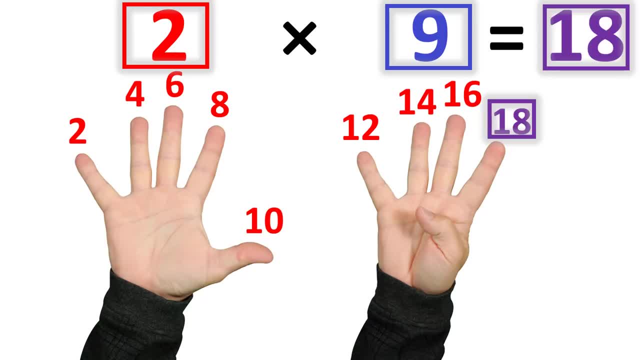 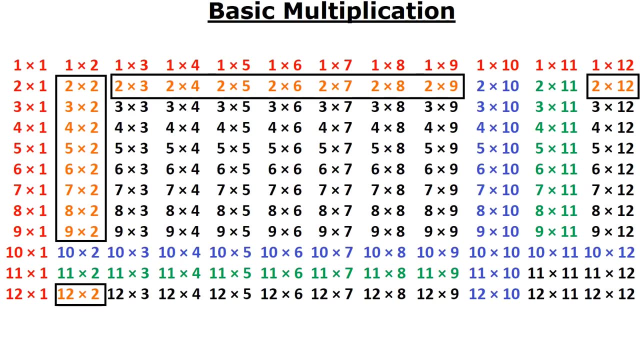 you stop at 18.. Because that's the ninth term. Very easy, right? Well, guess what? From those four rules, just four rules- you now know 77 math facts And you only have 67 remaining. It gets better. 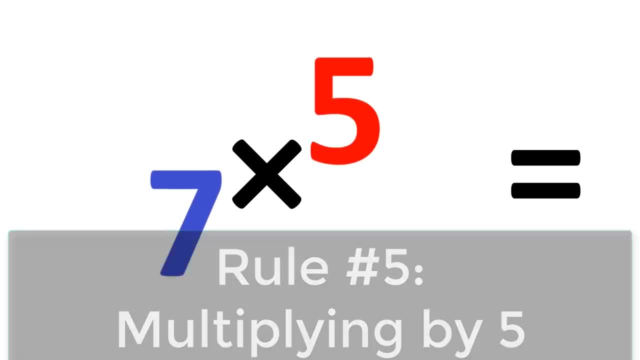 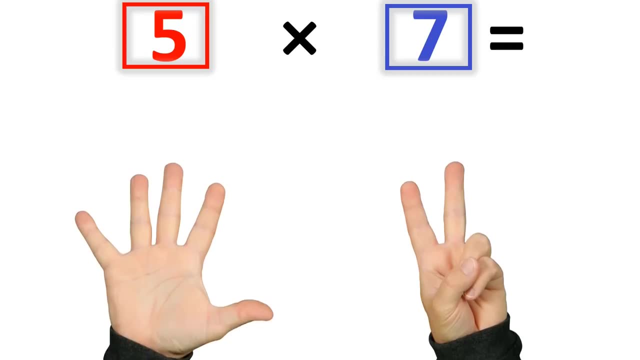 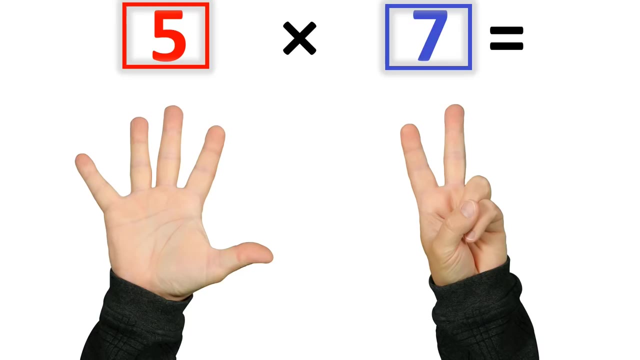 So for rule 5, we're going to look at the number 5.. And once again we're going to use skip counting, Because 5 is one of the easiest numbers to skip count by. So when you have 7 x 5, that just means you're counting by 5 seven times. So 7 x 5 just means you go. 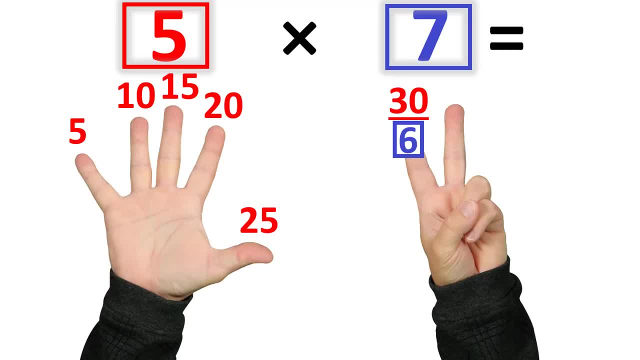 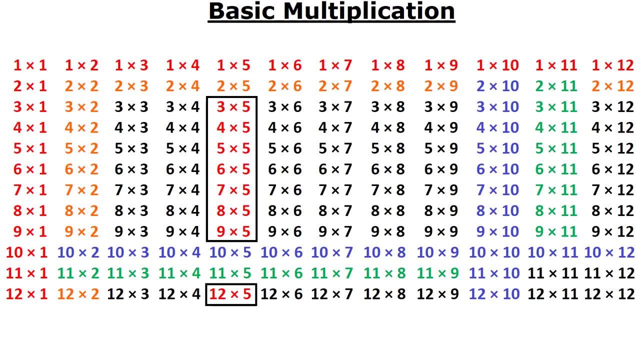 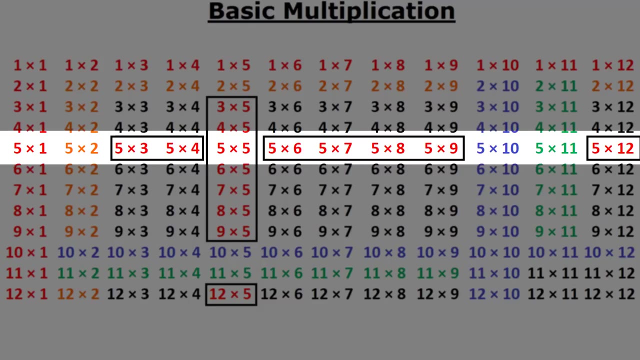 5, 10,, 15,, 20,, 25,, 30. And on the seventh one you stop at 35. Pretty simple, right? Well, now that you know 1 x 5 all the way to 12 x 5, that means you also know 5 x 1 all the way to 5 x 12.. So in total, 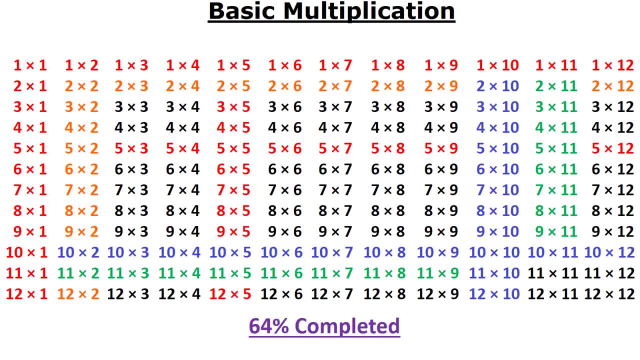 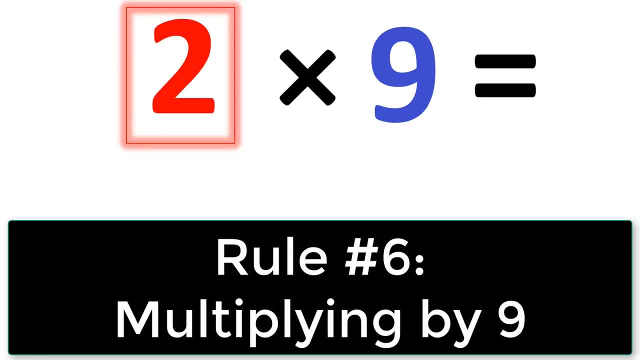 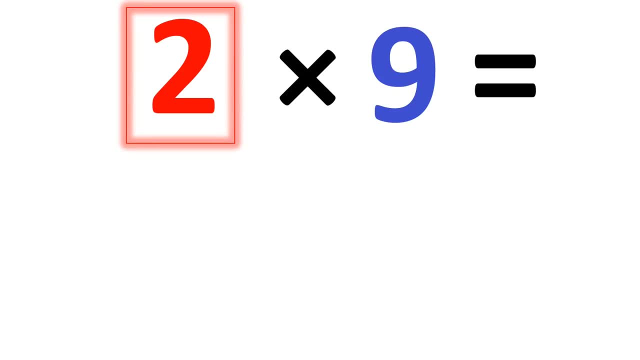 you now know 92 multiplication facts from just five rules, And there's only 52 remaining. So now for our last rule, Which is the rule of 9.. When you multiply a number times 9,, such as 2,, you take that first number, 2, and you take 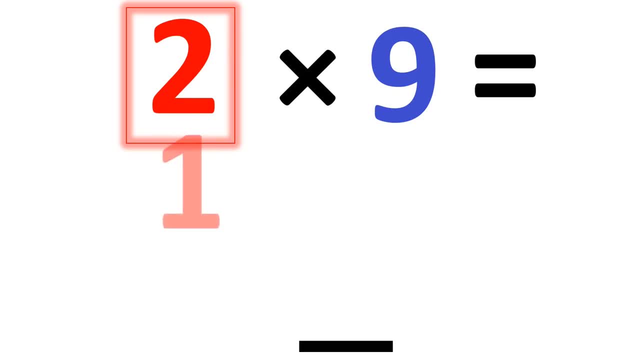 1 less than that number 2.. So 1 less than 2 is 1.. Then you say: 1 plus what number equals 9?? Well, 1 plus 8 equals 9.. So 8 becomes your second number. So the answer is 18.. 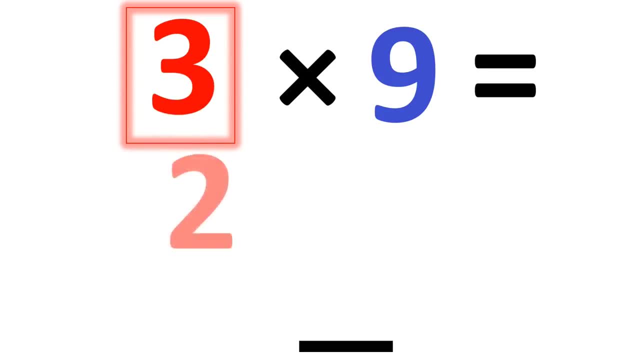 Or when you have 3 times 9, 1 less than 3 is 2.. Then you say: 1 plus what number equals 9? 7. So 27. So forth and so on: 4 times 9.. 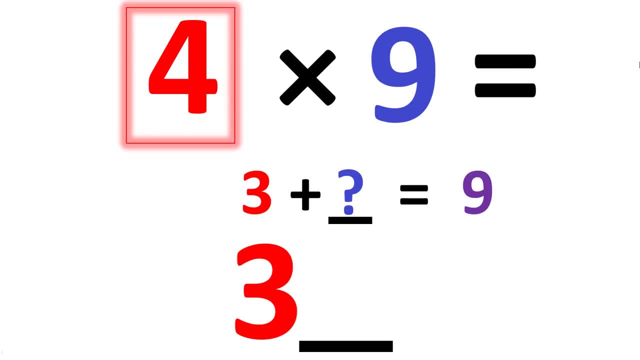 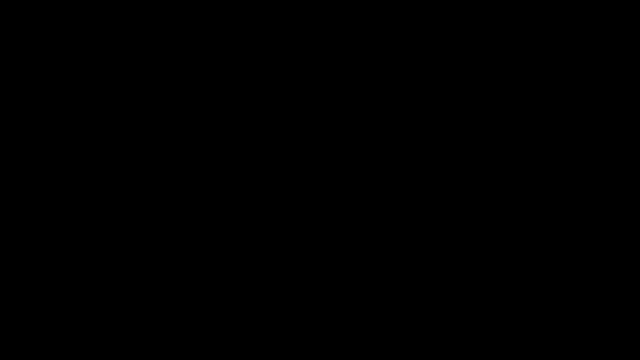 1 less than 4 is 3.. 3 plus what number is 9? 6.. So your answer's 36.. And you can do that all the way up to 9 times 9 to get 81.. So now that you know the answer to 2 times 9 to 9 times 9,, you also know the reverse. 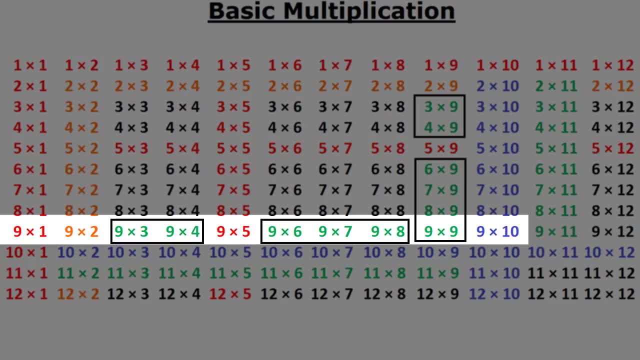 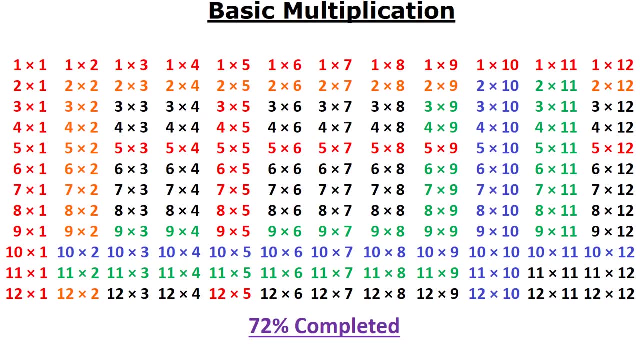 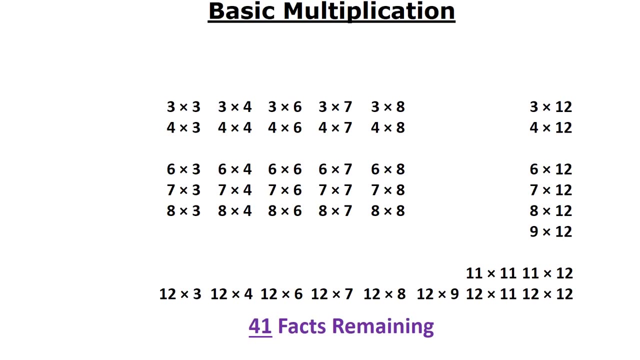 You know 9 times 2 to 9 times 8.. So, after just learning 6 rules, you now know 103 multiplication facts. That only leaves 41 remaining. And of those remaining 41, once we remove the duplicates multiplying by 3,, 4,, 6,, 7,. 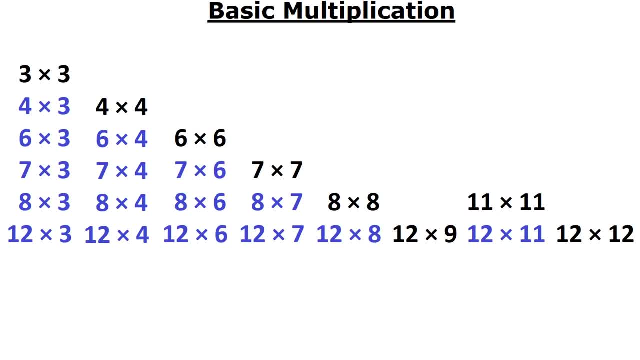 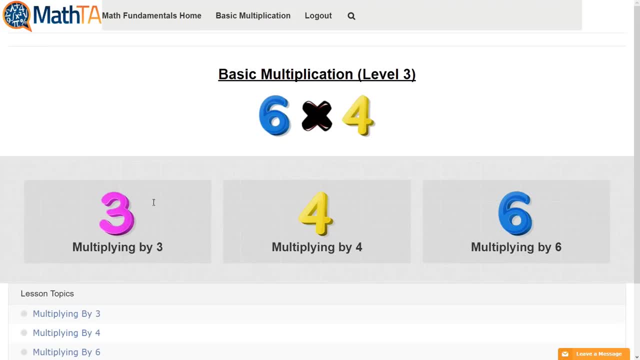 8, and 12,. we only have 24 facts remaining And you can learn those remaining 24 in record time. So now that you know the reverse, you know 9 times 2 to 9 times 8.. In addition to the 6 rules, we'll have daily practice, just 10 to 15 minutes a day, using 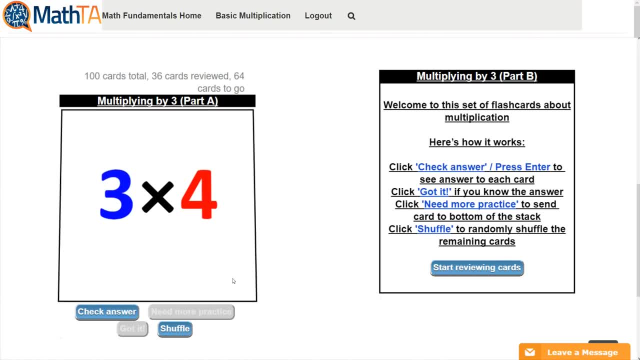 any computer, any tablet or phone. So what are you waiting for? Get started now.